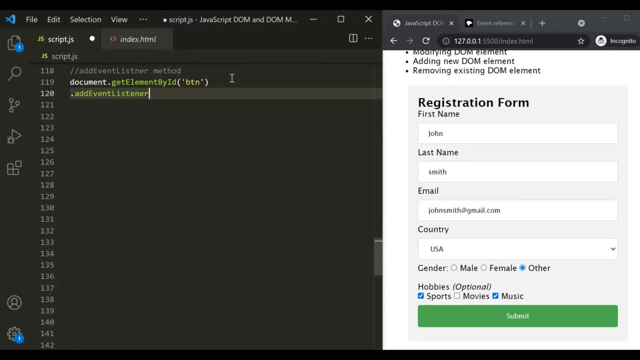 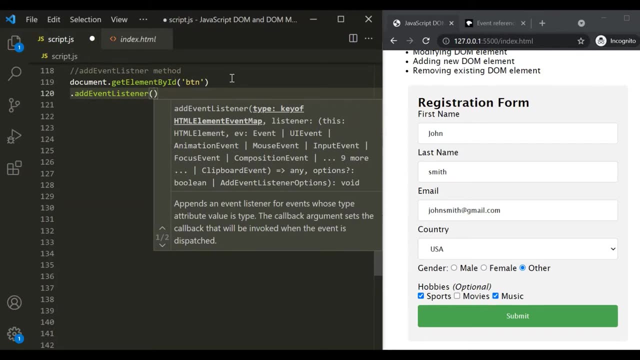 properties, But we are going to do this using add event listener method. Now this add event listener method takes two important parameters. First parameter is the name of the event which it should be listening to. So in this example, we want to listen to click event of this submit button. So as a first parameter, let's pass 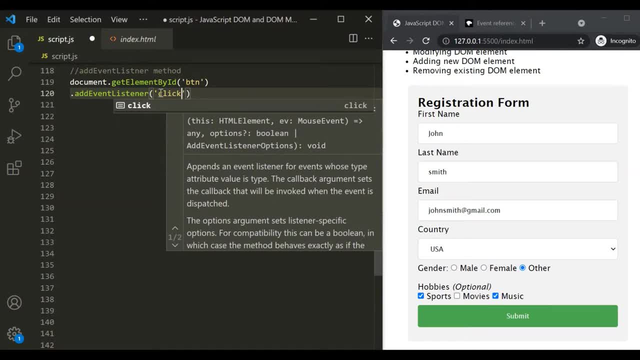 the event name, which is click Now. if you notice, here I am not prefixing this event with on, like we did for inline event handlers and event handler properties. In case of add event listener method, we simply pass the name of the event. Okay, we don't prefix it with. 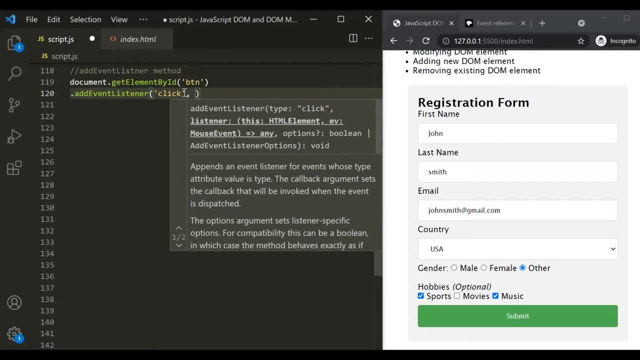 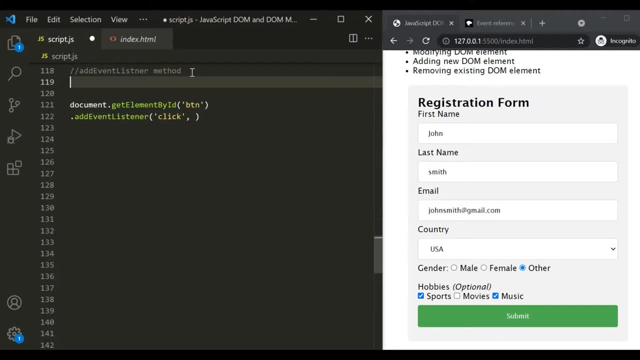 So let's create a function here. before this, you know, before we call this add event listener method, So let's create a function. let's call it display alert And, from within this function, let's call this alert function, which will display an alert window in the web page. 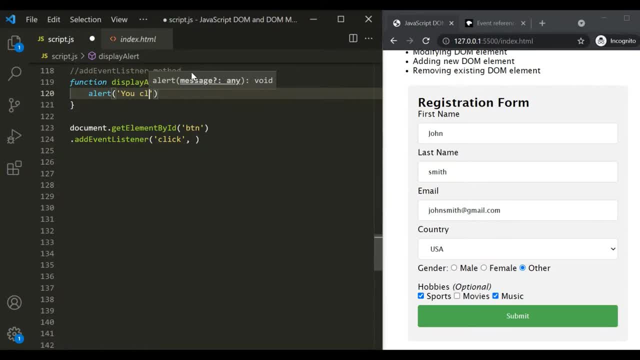 And what do we want to display here? Let's say we want to display: you clicked on submit button and that's it. Now let's pass this function as a callback function for this add event listener method. Now, if you remember, when we pass a function as a callback function, we don't use parenthesis. 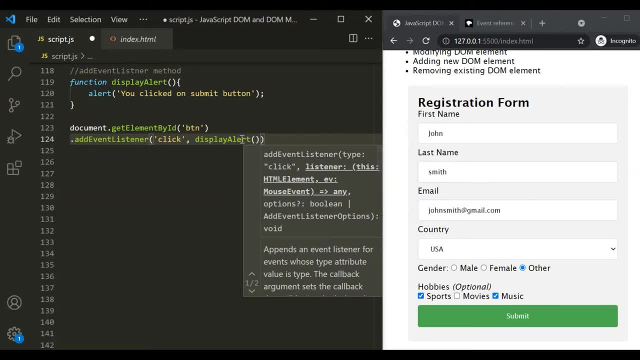 like this, because when we use parenthesis like this, it immediately executes that function, and we don't want that. We want this display alert function To be executed by add event listener function. OK, and when. it should be executed when this click event happens. So here we need not to specify these parenthesis. 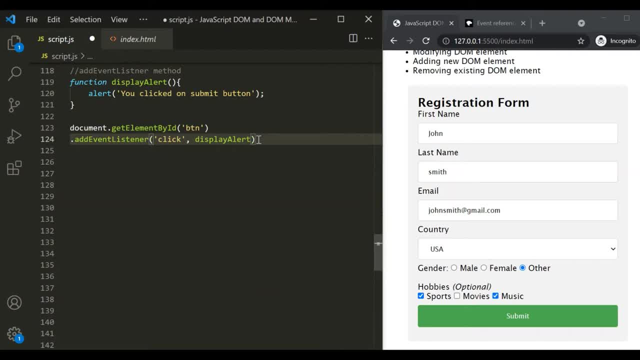 All right, And with this we have added an event handler function for the click event of this submit button. OK, Let's save the changes and let's click on the submit button and you can see an alert window has been displayed here. OK. 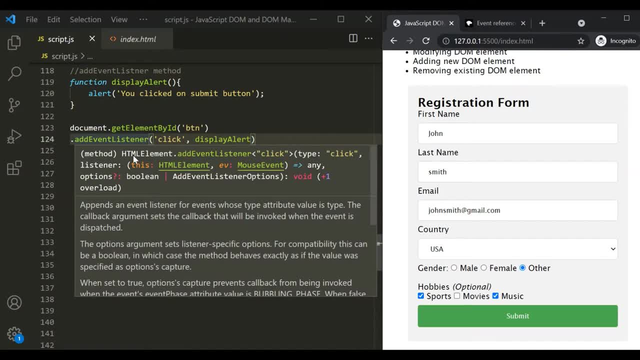 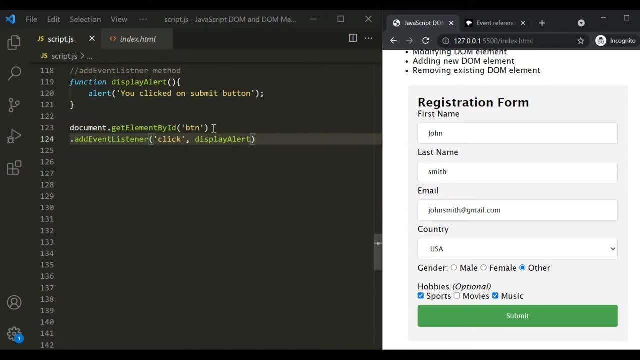 So this is how We use add event handler. I mean add event listener method. First we get access to the element on which we want to add an event listener and once we have access on access to that element, we use add event listener method to listen to. 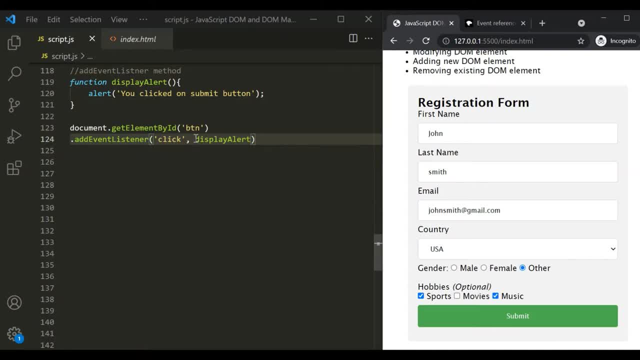 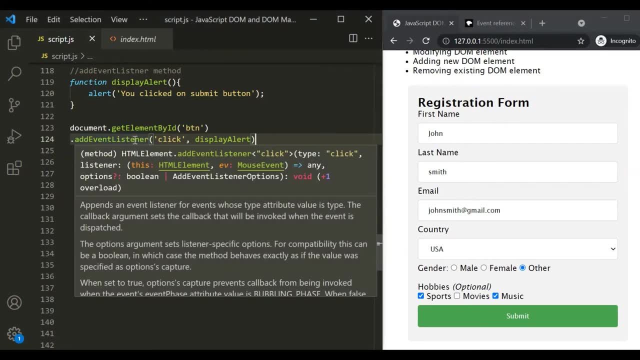 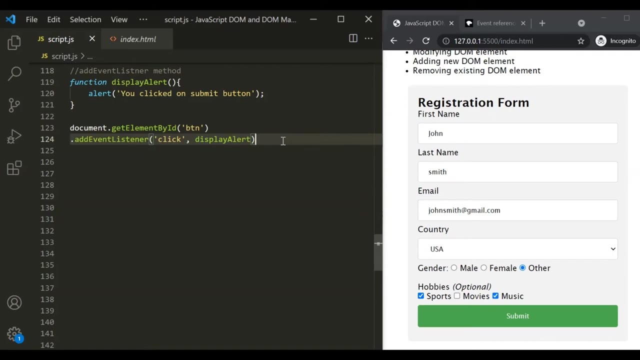 a given event and when that event happens, it executes the callback function. pass to it as its second parameter. Now, here for this add event listener method, We have passed a predefined function As its callback function, But it is also possible to pass an anonymous function as a callback function. 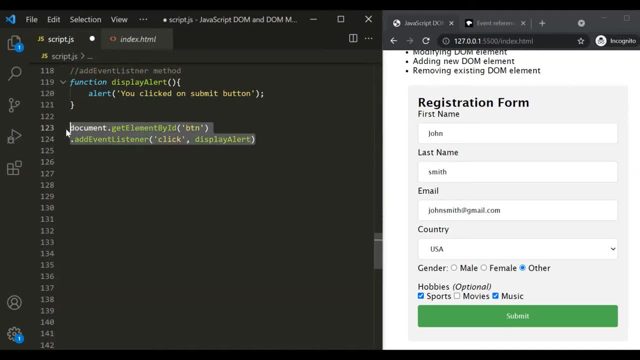 Let's see that. So again, let's copy this code here And let's comment this complete code. OK, So we are going to see how we can achieve the same thing using an anonymous function. OK, So now we don't have this display alert function. 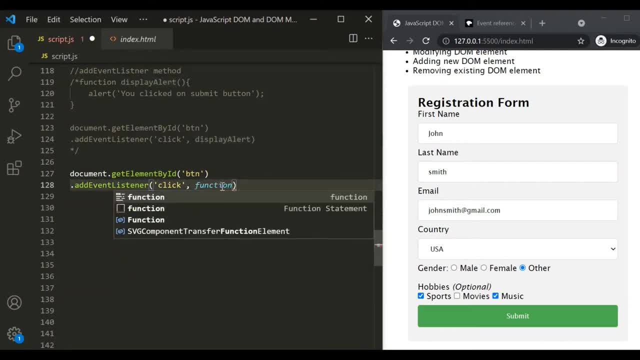 So instead of this, let's pass an anonymous function. OK, So now we don't have this display alert function. So instead of this, All right, And from within this anonymous function, let's call this alert function, And when this alert function appears, we want to display this message. 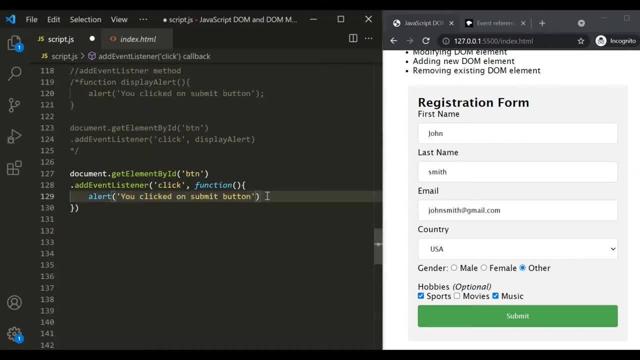 So let's copy that message, Let's paste it here, Let's save the changes, Let's click on this submit button. and it is still working as expected. So the only difference is here: instead of passing a predefined function, we have passed an anonymous function as a callback function. 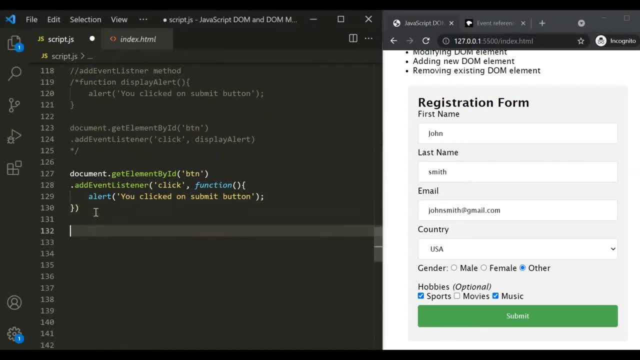 All right, Now let's use this addEventListener method to listen to other events. So here in this form, we have this email text box. Now what we want is, when we click inside this email text box, we want to change its background color to yellow. 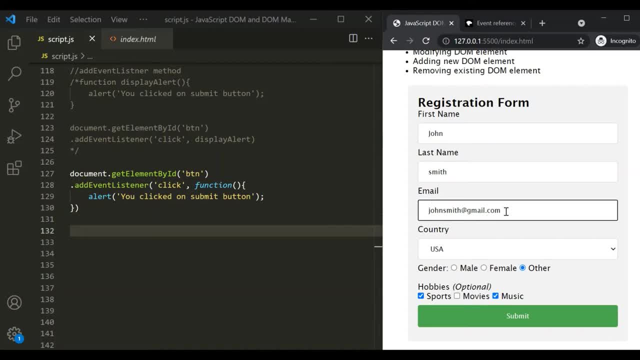 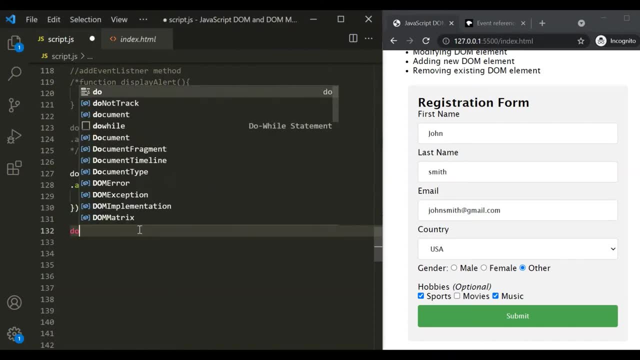 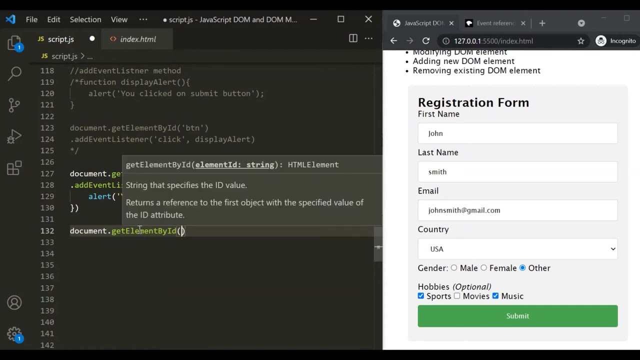 So here for this email text box, we want to handle focus event Right, So let's see how we can do that using addEventListener method. So first we need to get access to this element, This email text box. So let's say documentgetElementById, and to this we need to pass the id of this text box. 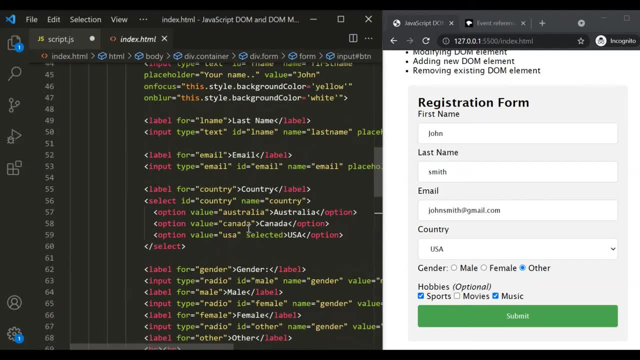 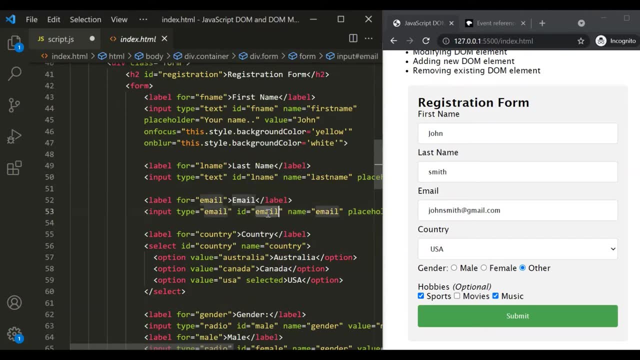 This email text box. Let's go to indexhtml again. Let's scroll up and somewhere we should have the email text box. So here it is Now let's copy the id of this email text box. Let's go to scriptjs. 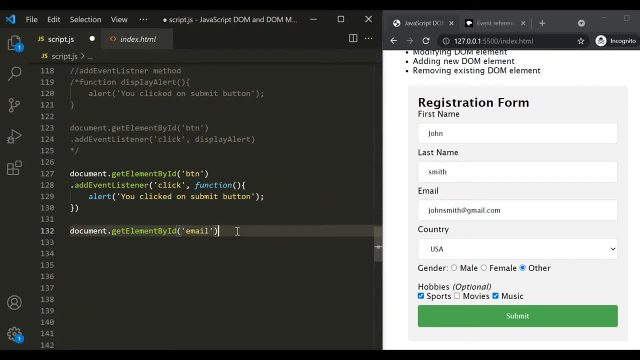 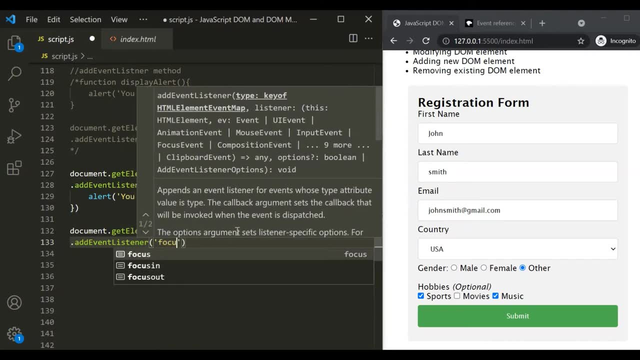 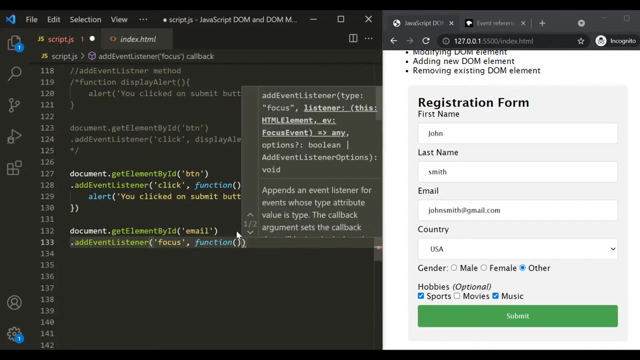 Pass it to this getElementById method and on that, let's add an event listener. Now this event listener should be listening to focus event, And when this focus event happens, we want to execute a callback function. Now, what should this callback function do? It should change the background color of this email text box to yellow. 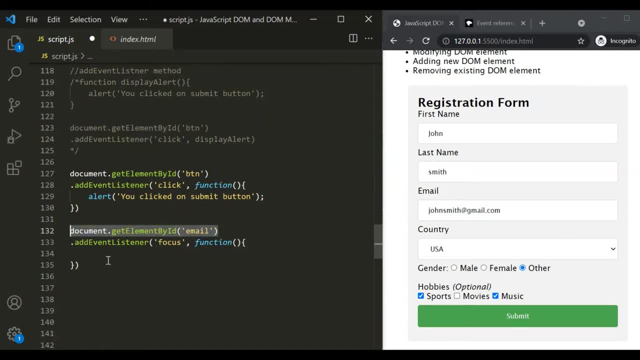 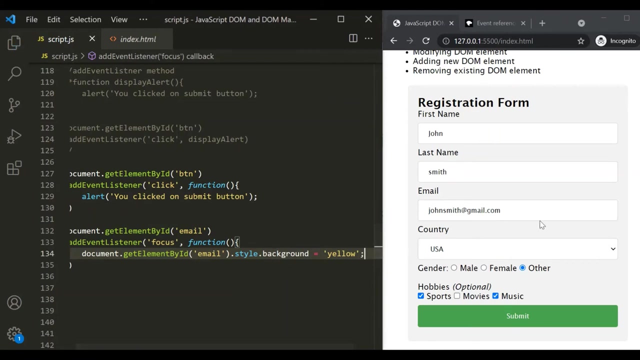 So again, let's copy this, Let's paste it here, And on this let's say stylegetElementById- Background And let's change it to yellow. Okay, let's save the changes. Let's click inside this email text box and you can see. now the focus event is working. 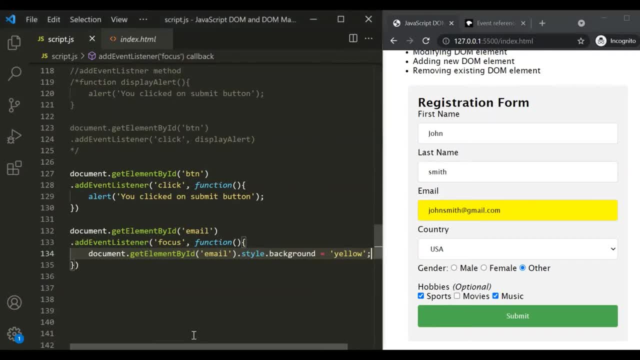 So whenever we are clicking inside this email text box, focus event happens, And when the focus event happens, this callback function gets executed and it changes the background color of this email text box. Alright, Now, if you remember, in the starting of this course, we learned that when we call a method, 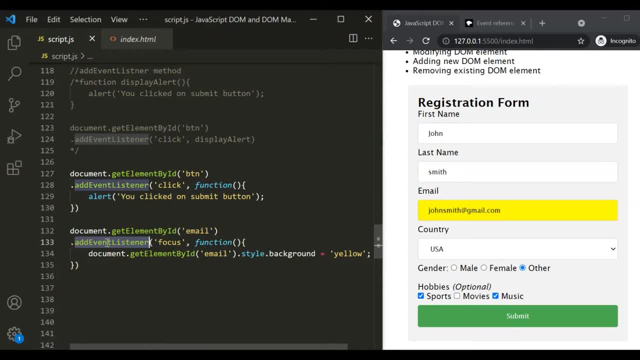 on an object, then inside that method this variable points to that object. Okay, so here we are using documentgetElementById method to get access to this email text box. Now in the DOM this email text box is stored as an object. Okay, So let's say documentgetElementById. 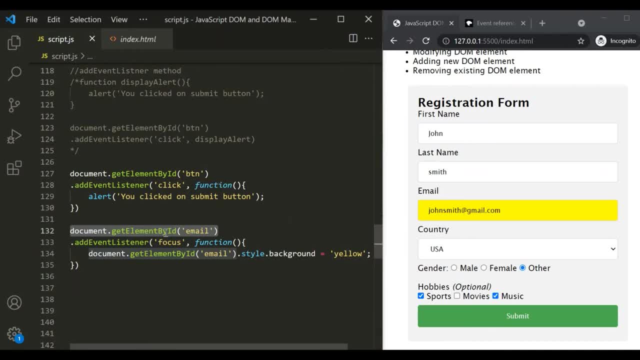 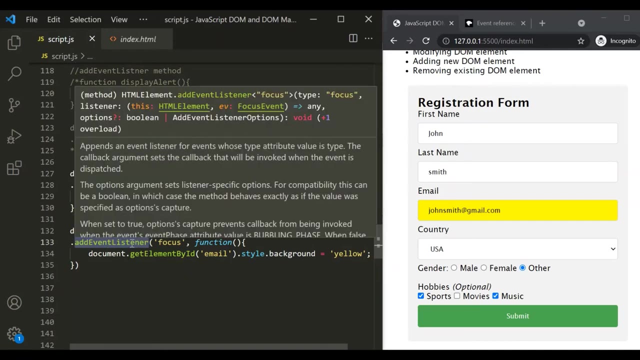 And when we pass this id of this text box to this getElementById method, it is returning us a DOM object And on that DOM object we are calling this addEventListener method. right, That means, inside this addEventListener method, this keyword will point to this DOM object. 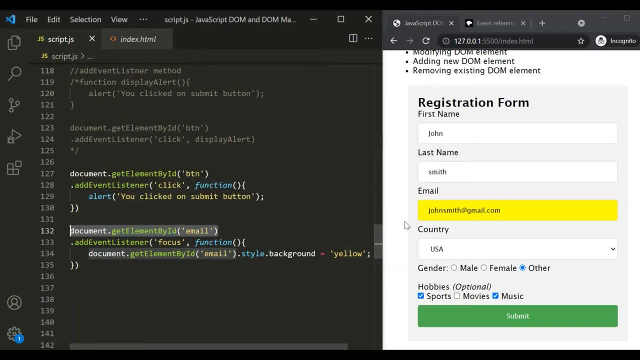 which this documentgetElementById method has returned. That means it has returned this text box. So inside this addEventListener method, this variable will point to this text box. So instead of writing this complete line of code here, this documentgetElementById, we can also simply say this: dot style, dot background. 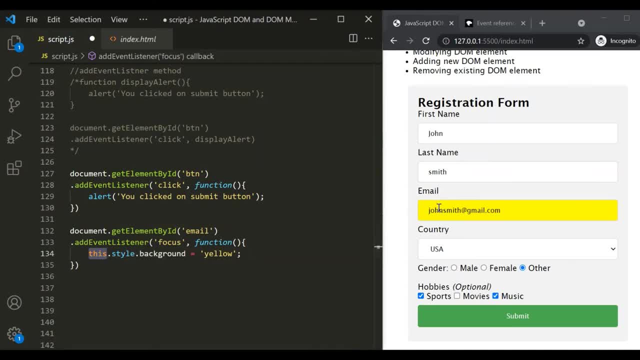 So here this variable is pointing to this email text box. Okay, Let's save the changes and let's see if it works as expected. So if I click inside this email text box, it is still changing the background color to yellow. Now just to check where this keyword here is pointing to, let's log this keyword in the 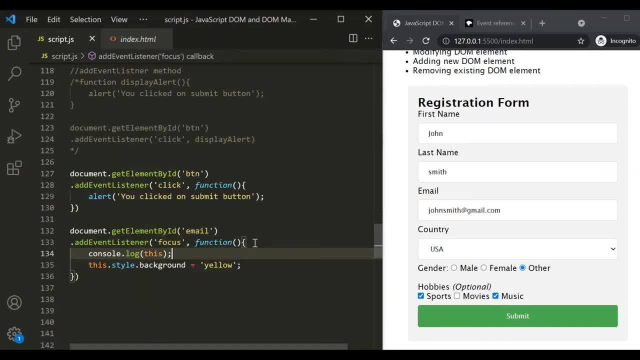 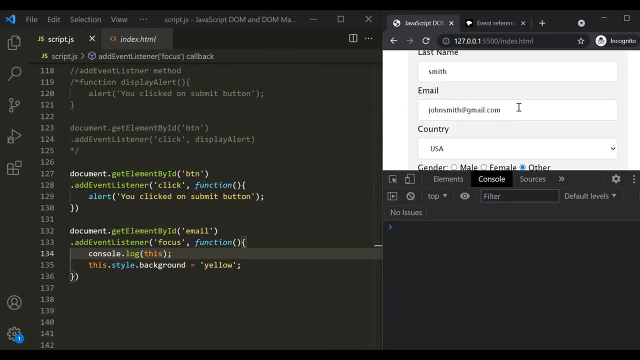 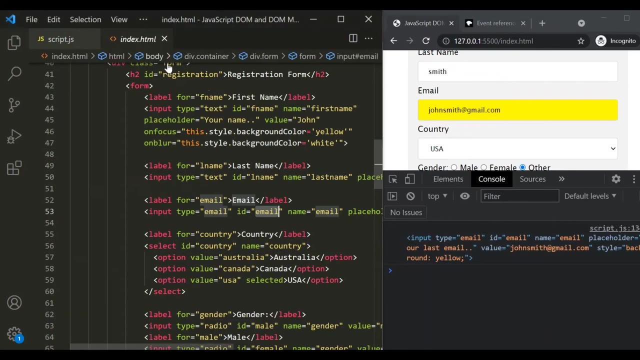 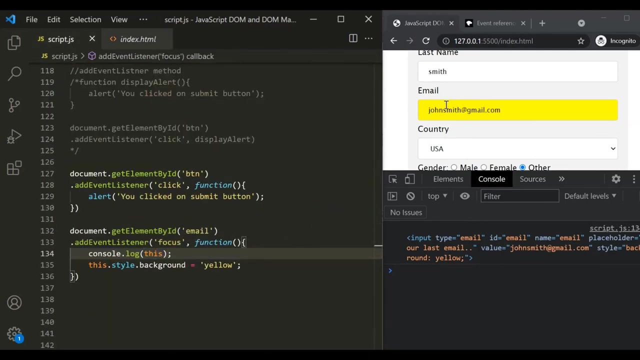 developer console. Let's save the changes. Let's open developer console here and now. let's click inside this email text box And you can see it has logged that same input element, This input element. So here this variable is pointing to this email text box. 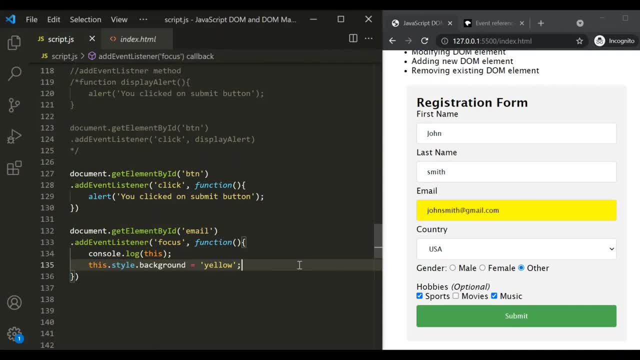 Okay, all right. So this is how this addEventListener method works. To the addEventListener method we pass the event, The event name which we want to listen to, and when that event happens, we pass a second parameter- You know, a callback function- as a second parameter which gets executed when that event happens. 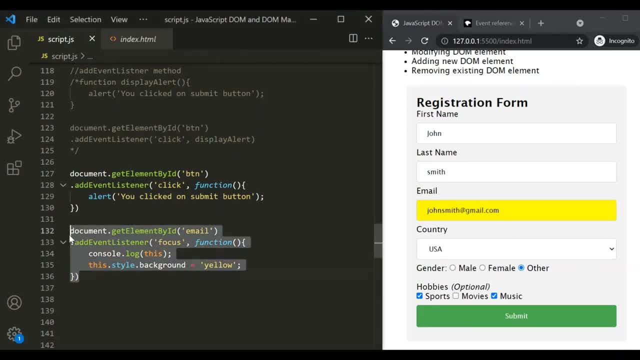 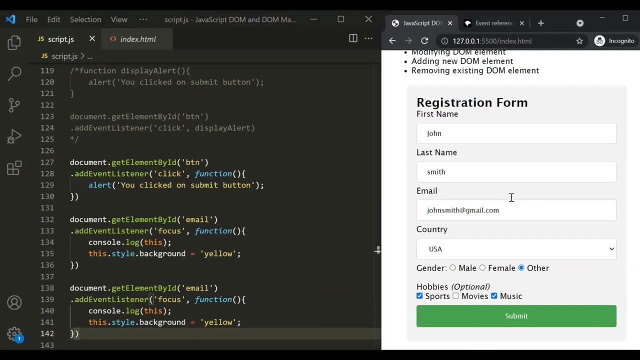 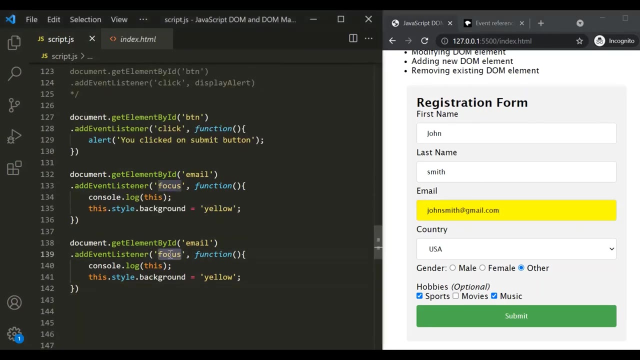 So here we are handling this focus event. Let's also focus. I mean, let's also handle the blur event, So that when this email text box loses its focus, its background color should change back to white. Okay, So now we want to handle blur event. 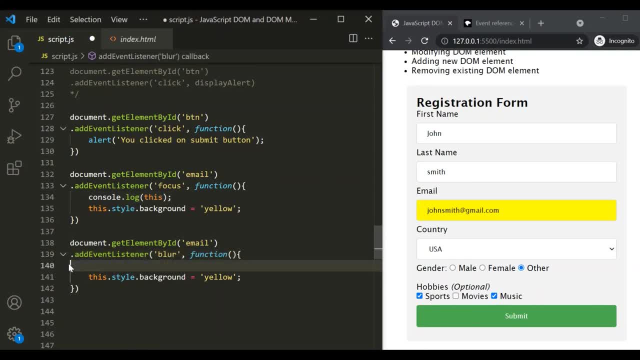 Okay, And let's remove this consolelog statement from here And let's change the background color to white. Save the changes. When I click inside this email text box, it is changing its background color to yellow. When I click outside, it is changing back to white. 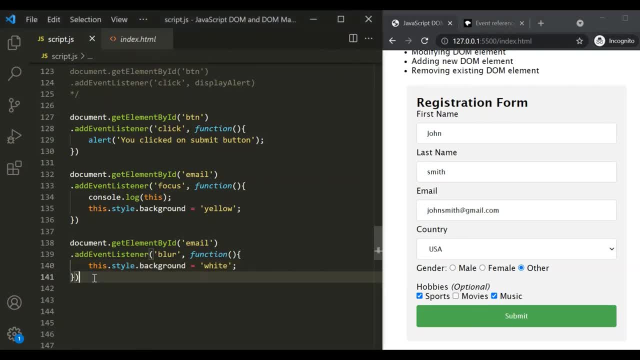 So here we have handled the blur event as well. Okay, so this is how we can handle events in JavaScript using addEventListener method. And remember that out of inline event handlers- Okay, EventHandler properties and addEventListener method, This addEventListener method is used mostly and the inline event handlers are used least. 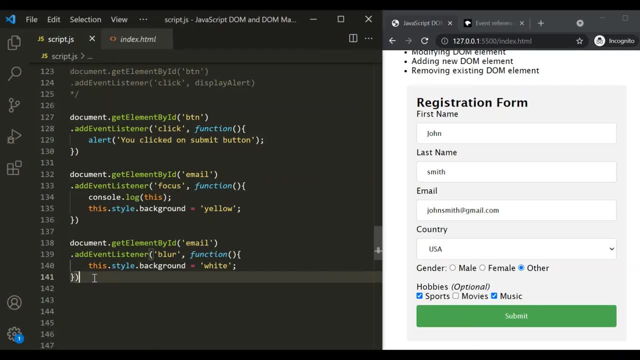 This is all from this lecture. In the next lecture, we will learn how events are executed behind the scene. Thank you for listening and have a great day.